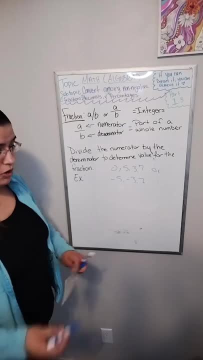 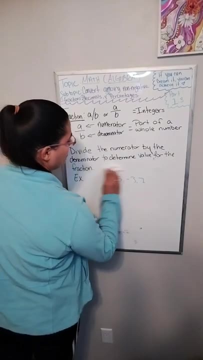 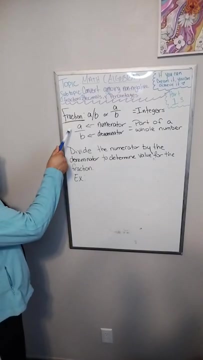 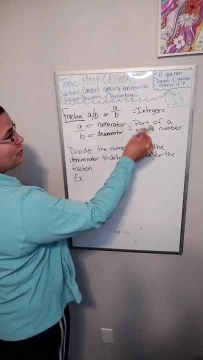 negative three negative seven. those that's what integers are. okay, a numerator, like i said, is the top of the number, the top of the fraction, and the denominator is the bottom of the fraction and this will equal part of a whole number or an integer, part of a. 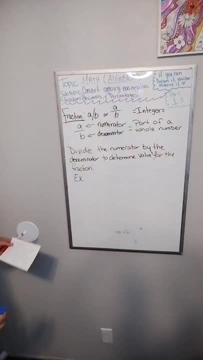 whole number or an integer? okay, we will. in order to find the fraction? in order to find the fraction, we would have to divide the numerator- the numerator, this one, by the denominator here, this one, for it to give us the fraction. okay, and it's very important that you. 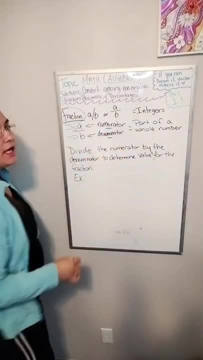 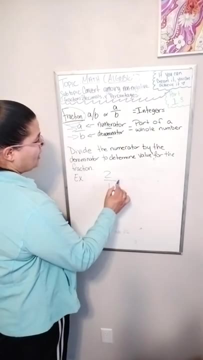 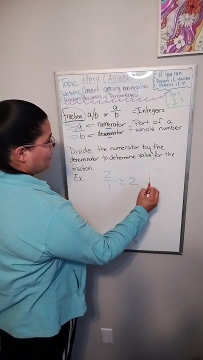 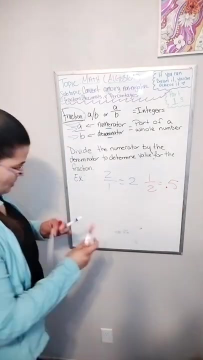 divide the top number by the bottom number, not the bottom number by the top number, because it will give you a different result. for example, two divided by one is going to give you two. one divided by two is going to give you your fraction at point five. okay, all right, let's delete this again. 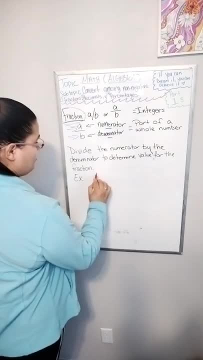 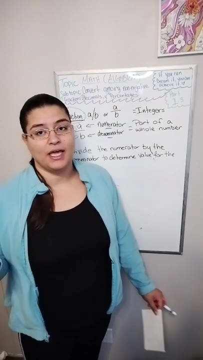 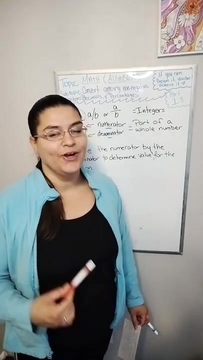 so other examples. to go bigger, it's going to be 36 divided by 11.. 36 divided by 11. on the t-s test, you will have a calculator so you can just input this on the calculator, just like this. i am not going to go over the work this test becomes. 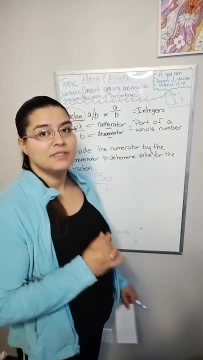 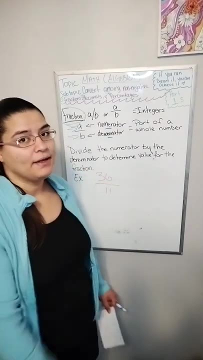 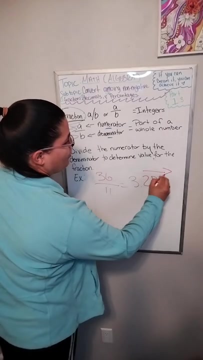 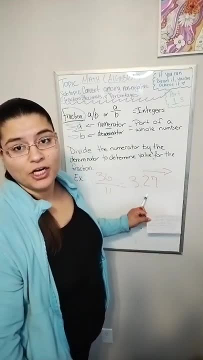 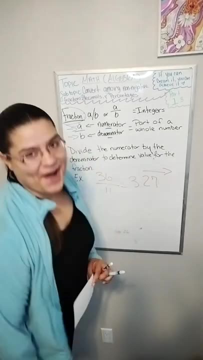 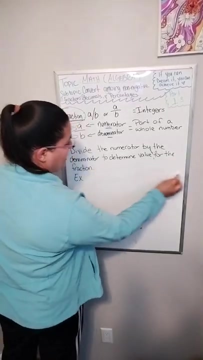 give you somewhat of a hard one, because when we're learning chemistry, you're going to see this one again and how we can work this problem later. okay, but for now i just want to uh, dip your toes in, like one would say okay. so one more example in order from, and and we can cut this video off.